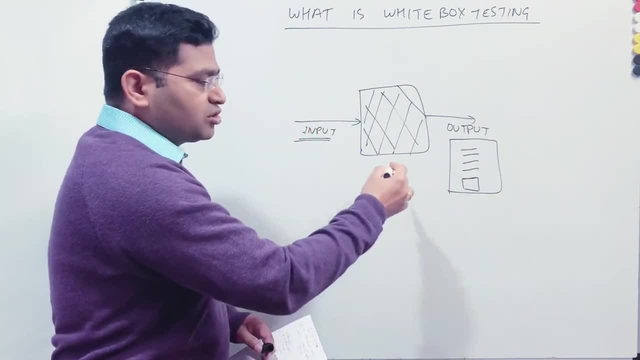 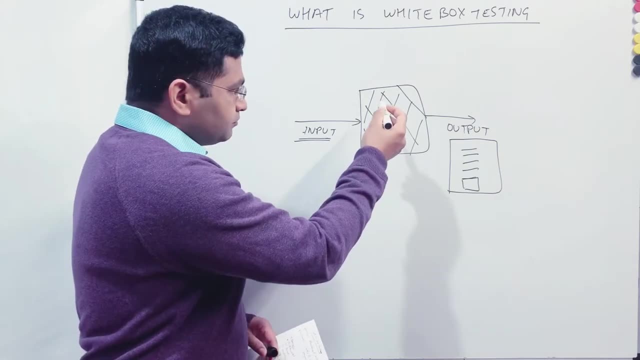 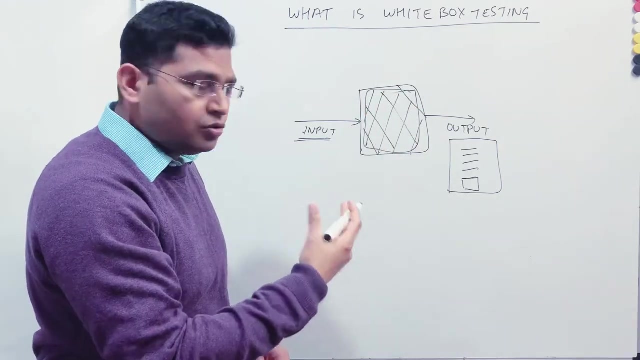 opening successfully or not, right. So this is black box testing for me. Now, when we talk about white box testing, white box testing is concerned about what actually happens within this box, right, Or in the actual code. so say, for example, if I click on register link, I need to have 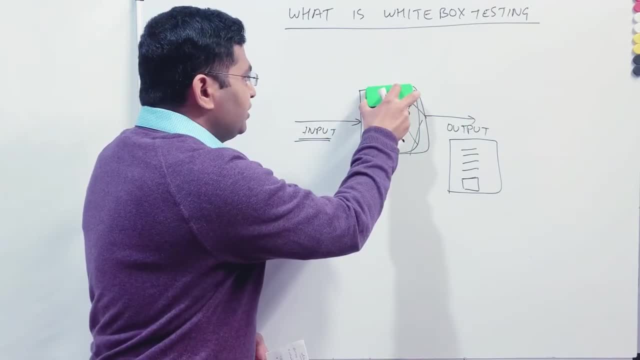 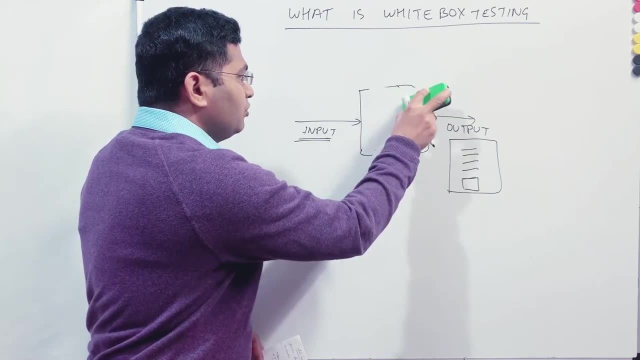 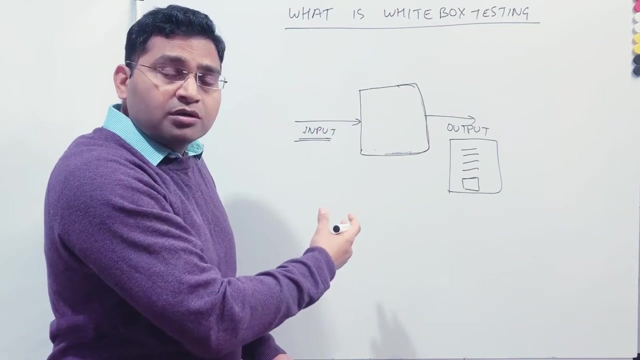 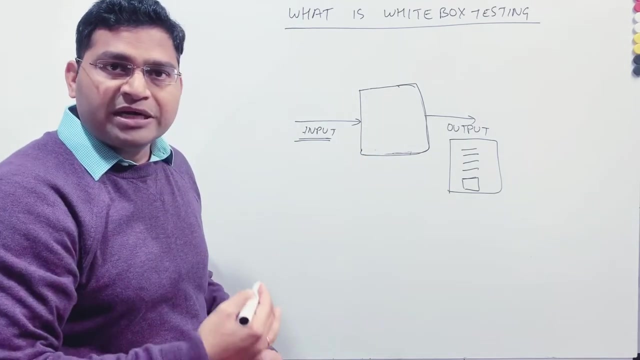 understanding of what all happens within the code which is being written for that particular functionality. right? so, before this registration page is being displayed, what all methods are being called, what all classes are being written. so, depending on which programming language you choose, what implementation has been done by the developer? if I am concerned about the 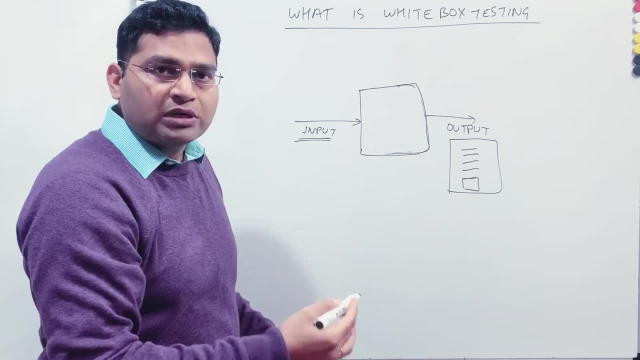 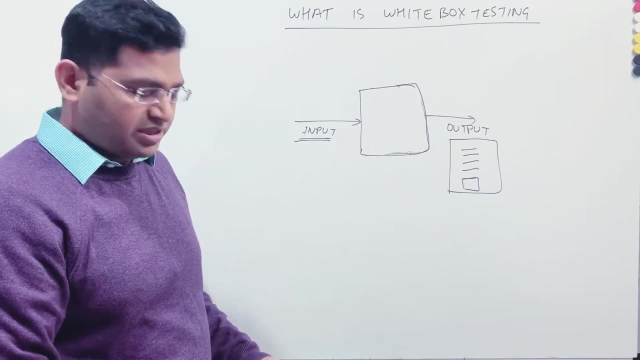 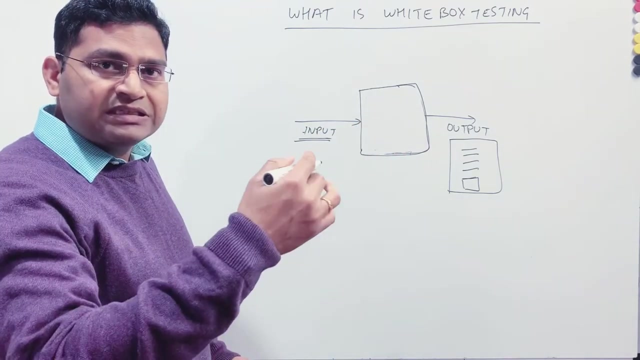 details of those implementation, then that is known as white box testing. white box testing is also known as glass box testing, clear box testing or structural testing. right, so when you check the structure of the code, so it's in in the structural testing. there are many types of white box testing which we will cover. 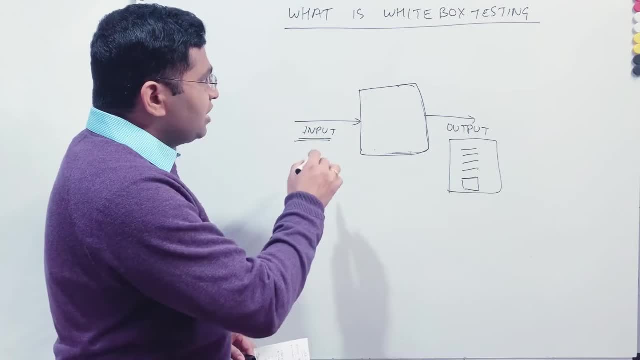 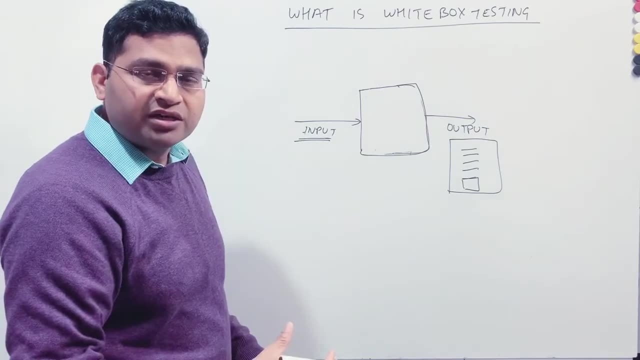 in detail in upcoming tutorials, but as of now, you can see that the code is being written and the code is being written in. just understand, when you are deep, when you want to understand the internal working, how the code, how the methods are written, which methods are which class. 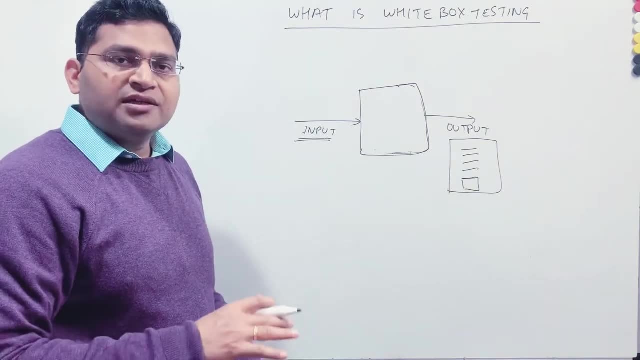 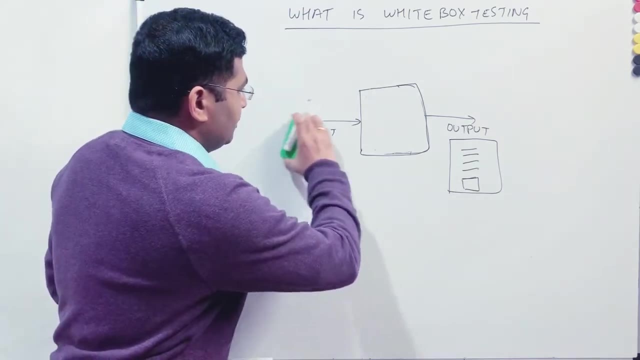 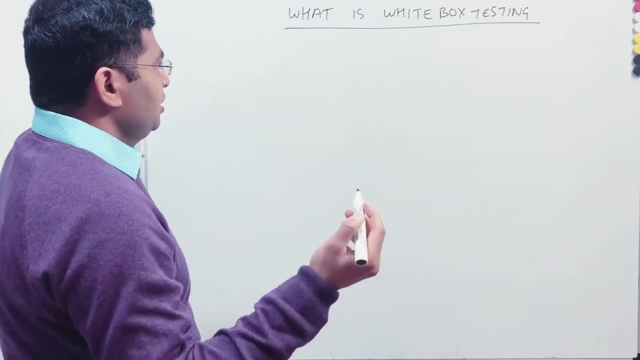 calls which car class, so all that details. when you are trying to test, then that is known as white box testing. now let me take an example of white box testing and I'll explain. you know how you can explain the white box testing to the interviewer. now say, for example: I'll take very simple example of calculating. 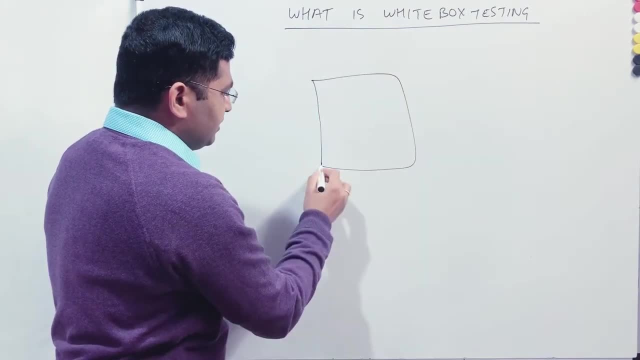 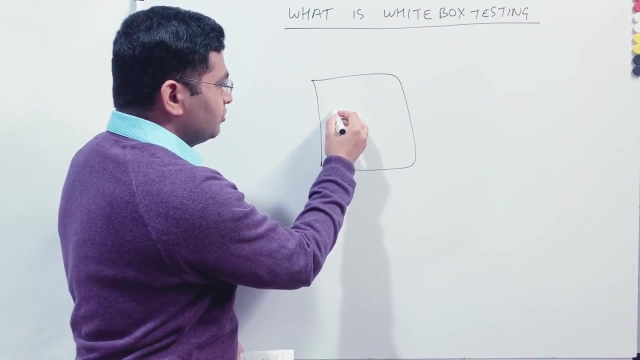 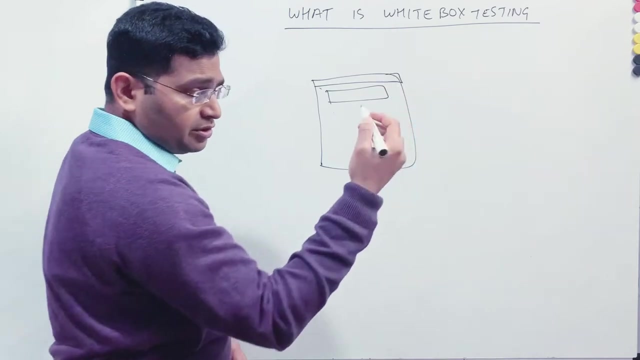 okay. so, for example, there is a website, all right, and on the website you have the calculator. so usually what you'll do is you have certain you know like numbers there, so you have the screen and you have if you are accessing the calculator on the website. so there will be some screen and the daily you know like. 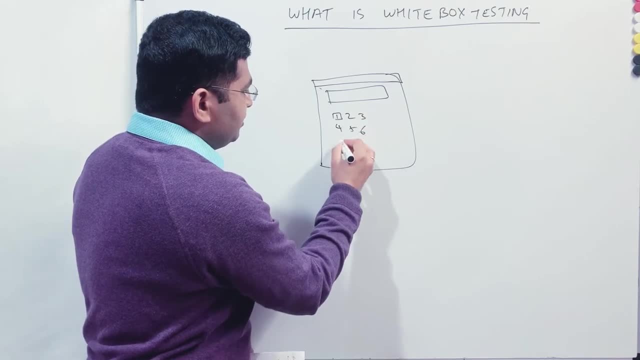 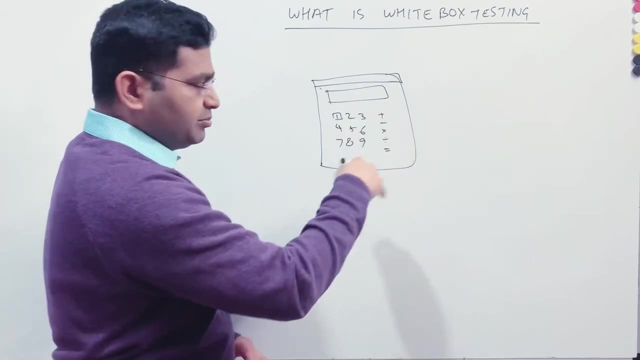 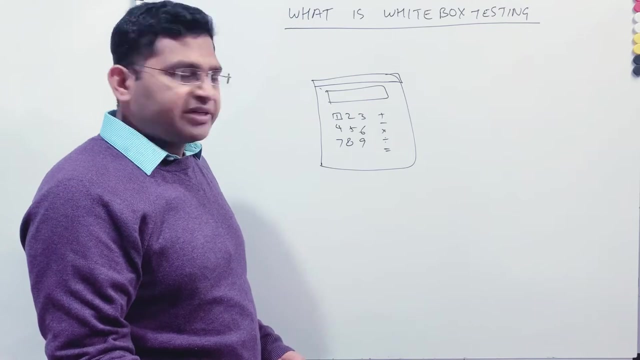 certain numbers: one, two, three, four, five, six, seven, eight, nine right, and then plus, minus, multiplication and division and equal to sign. so very simple. so, for example, I've taken the calculator. so if you are trying to test the calculator using the black box technique, what you will do is, if you want to, you know, test all the functionalities. you will test the. 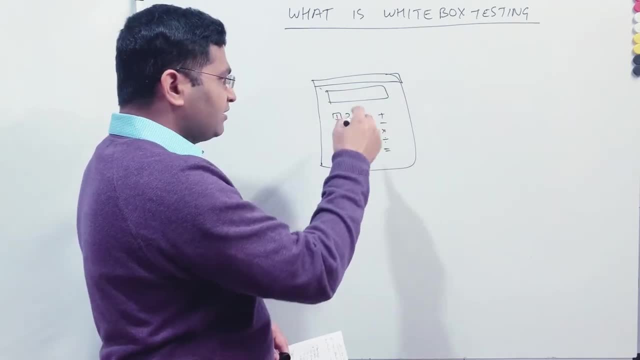 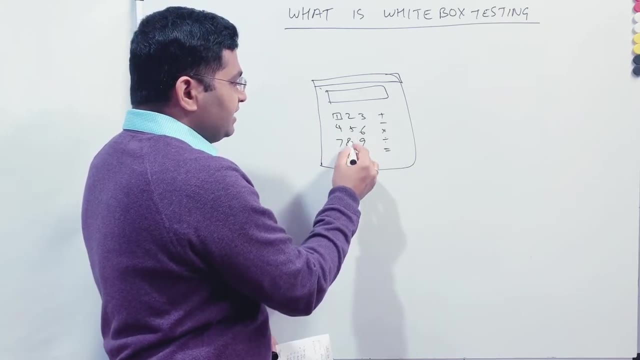 addition, subtraction, multiplication and division. right, so this is simple calculators. what I'll do is I'll try a couple of scenarios with the addition. so I'll say seven, I'll press seven and then plus eight, and then I'll verify, press equal to and verify that the sum is what I expect. 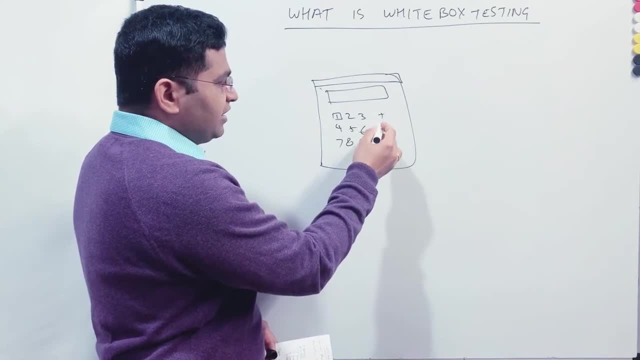 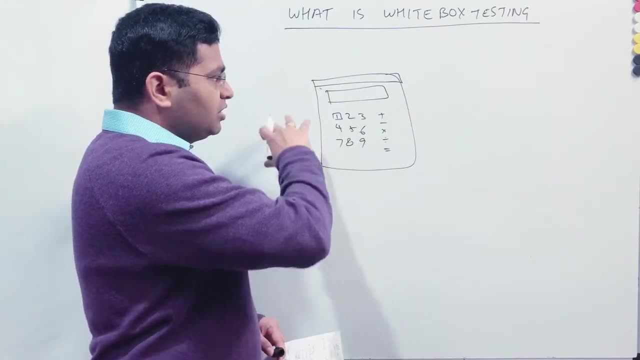 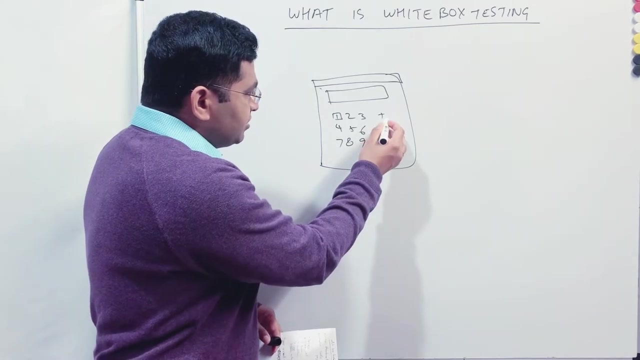 okay. Similarly, if I want to verify the subtraction, I will follow the different scenarios or the test cases to verify those scenarios. so this type of testing will be the black-box testing for me, because once I press seven and then press plus, and then press eight and equal to, I am. 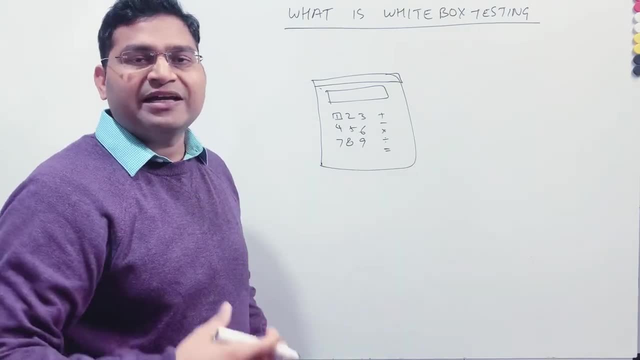 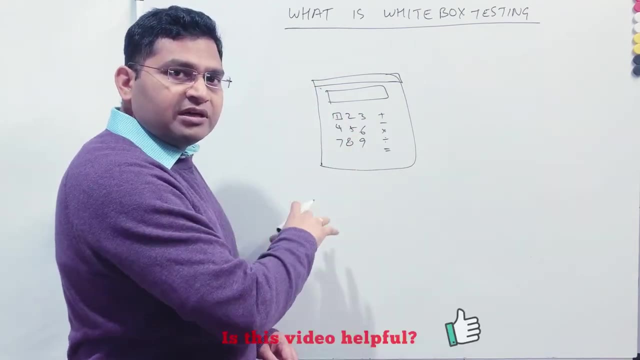 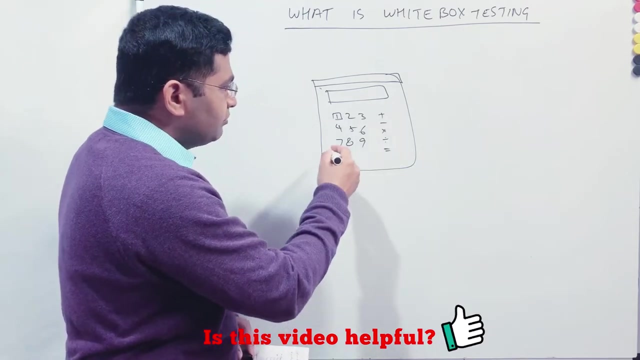 not concerned how internally that calculation is happening. okay, so the internal of this particular calculator, I don't know, and that is why this is black box for me. When I talk about the white box testing the same calculator, basically, what I'll do is I'll open the box, right. 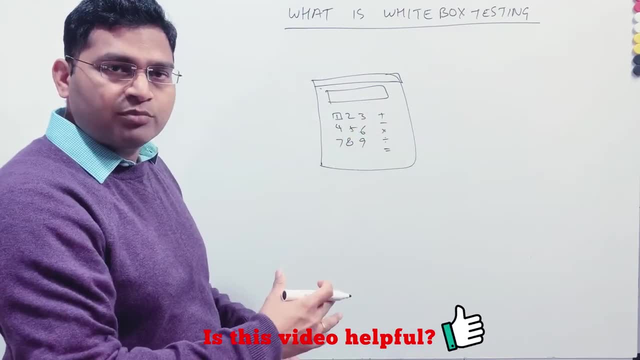 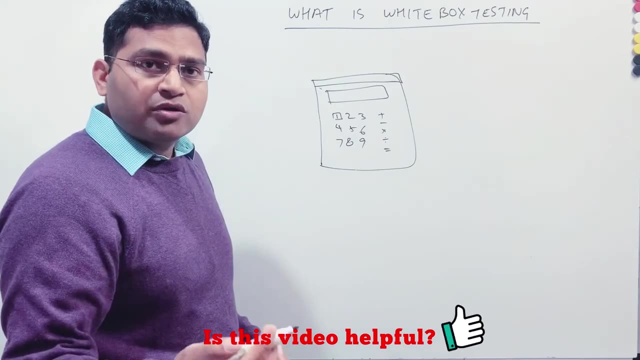 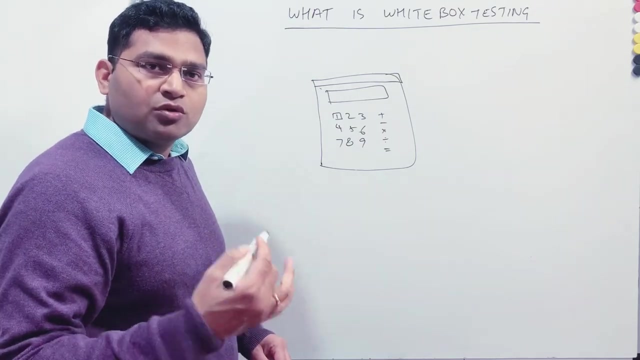 so as it says white box and black box, so in the white box the box is open or it's not a black box for me. I know the internal working or I need to know how the actual calculation happens. so in the white box testing you will mostly work with the actual code, right. so in that particular case 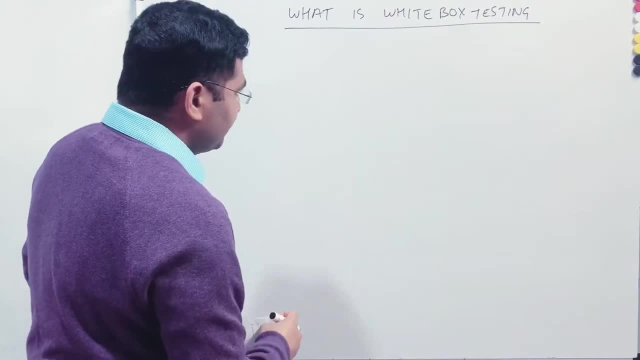 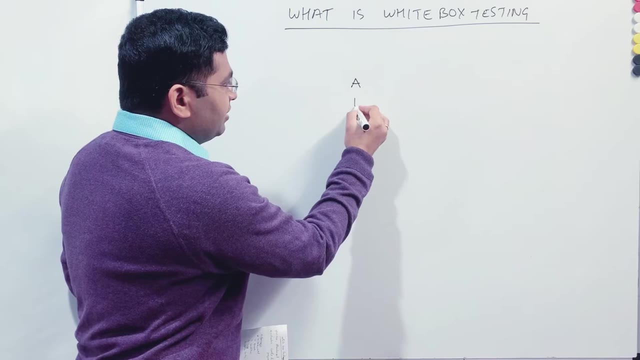 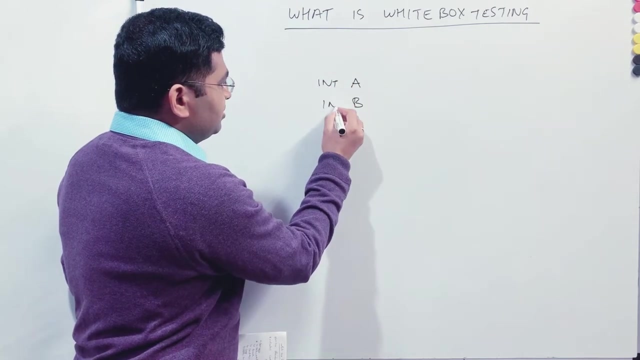 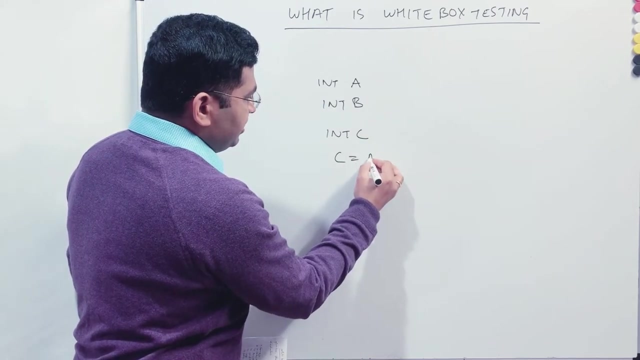 what you will do is say, for example, I'll write some pseudo code here, so I have an, a number a, a number b, and then say, for example, this is integer integer. and then there is another integer, c, and c is equal to a plus b, and then basically return: 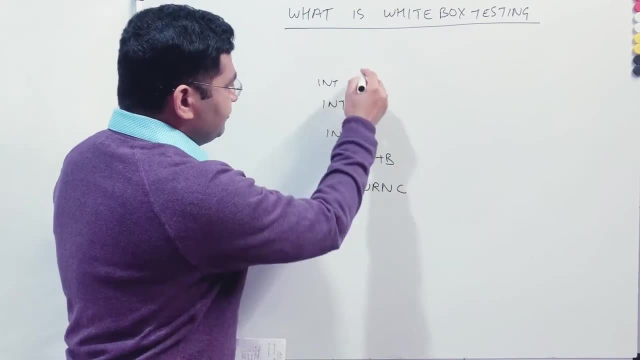 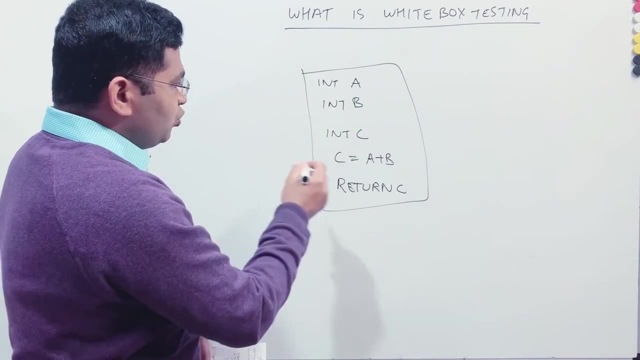 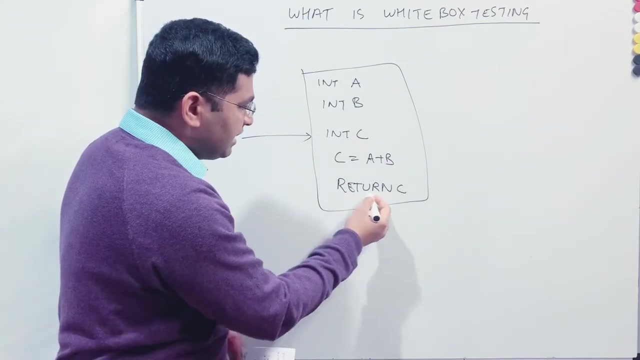 c. So, for example, this is one of the addition method that has been implemented as code, right? so if it is white box, then I know that this is what the code has been written for the additional functionality. Similarly, I'll have access to the code that is implemented for the. 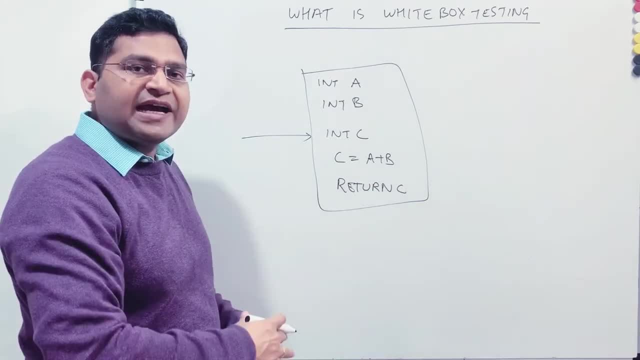 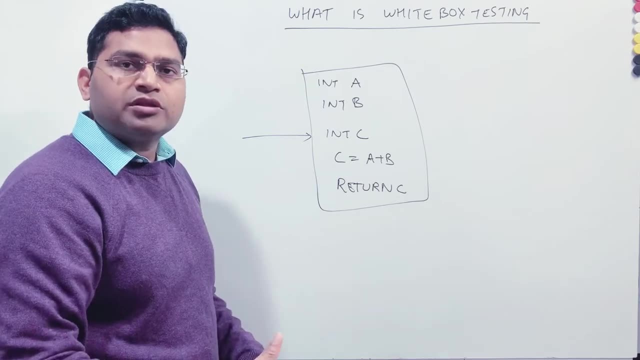 multiplication, for division and similar will be the case in the actual application. So I'll check it out. So what I'll do is we have these integrating applications. So, as you can see, there will be not only the code, but there will be other applications for equality or respect. 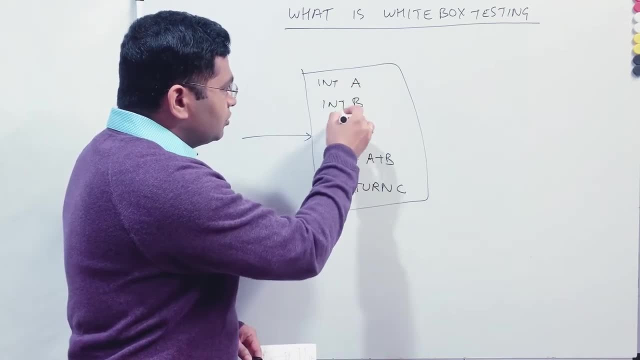 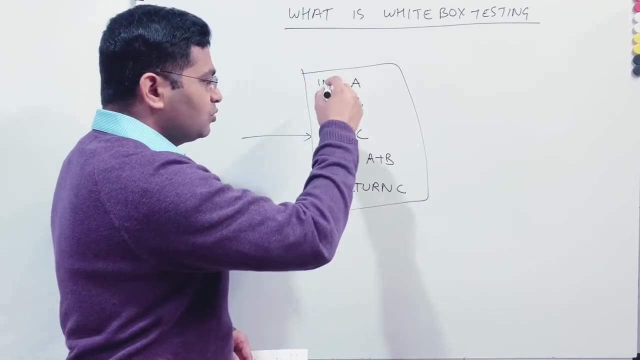 for the application. So again, they all are going to be defined and we are asking for the code over to students. let's say goodness me why I got says that right here in English. Let's go and I'll click the test and notice that right now they are coming out. I have got a lot of 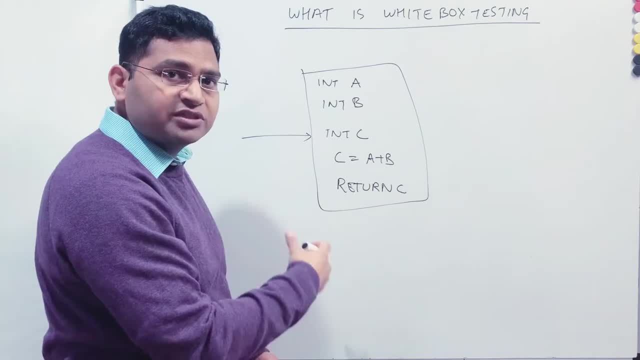 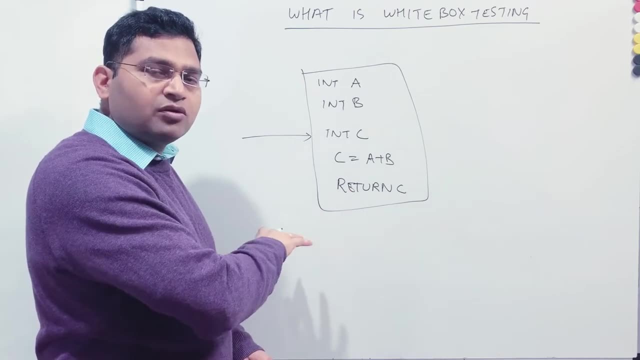 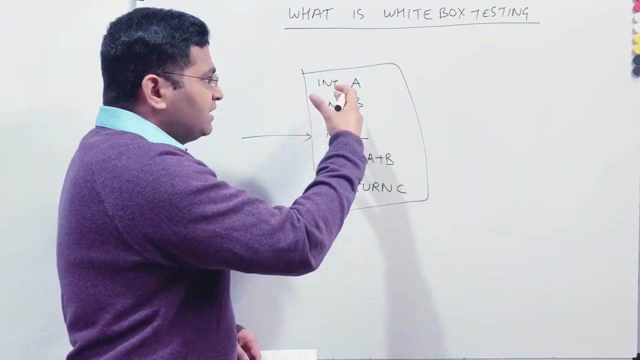 this particular you know code with valid values, invalid values, so i'll try with float, i'll try with you know invalid numbers, i'll try with with passing all other you know negative scenarios and see how this particular code behaves, whether it just accepts integers and returns the integer. 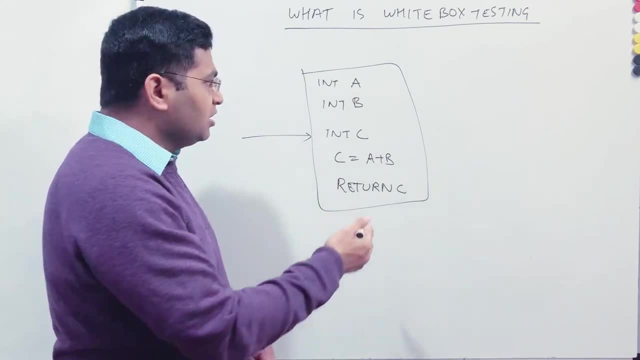 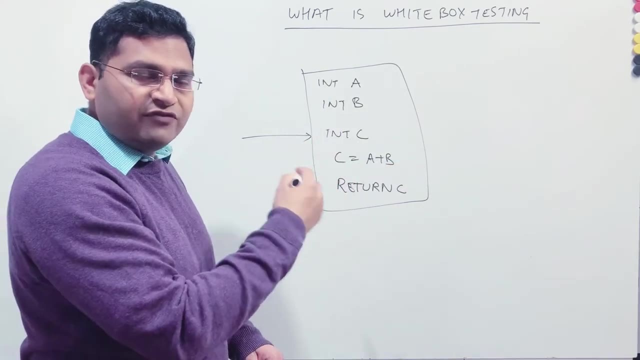 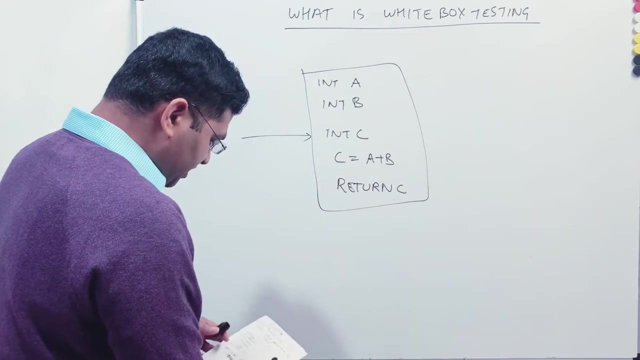 you know sum or multiplication, etc. or it crashes if i provide some invalid value, right? so when you do this type of you know verification, then that is white box testing, and in white box testing there are many techniques. so basically statement coverage. so there are many types of testing. 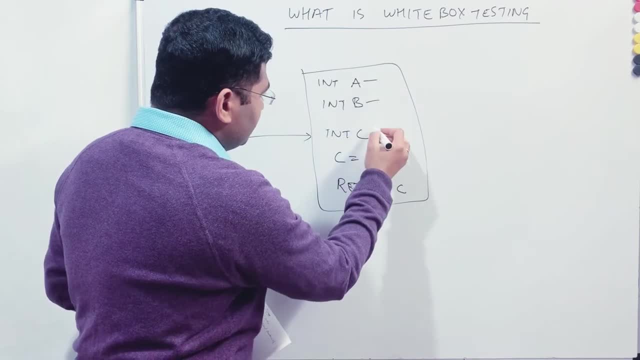 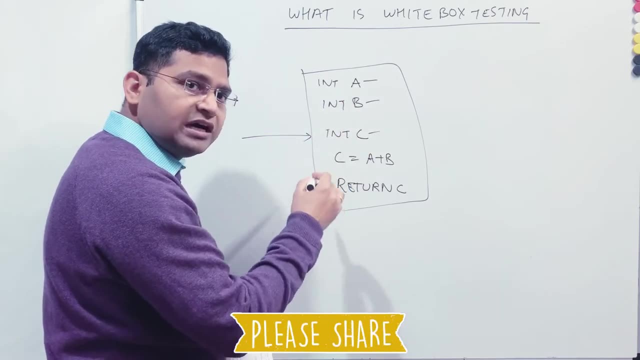 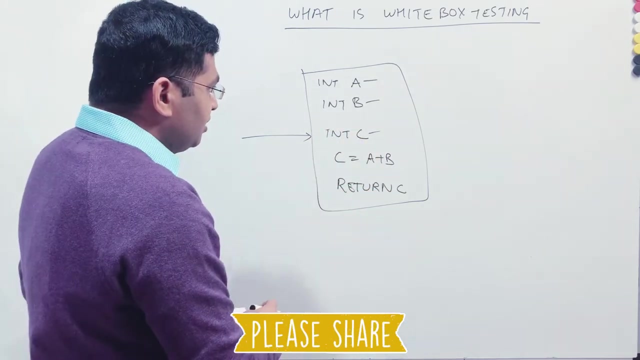 so the statement coverage, when you cover each and every, you write the test case so that you verify that the statements, all the statements in the code, are being covered. that is known as statement coverage. then you have, you know condition coverage, loop coverage, and then you know like: 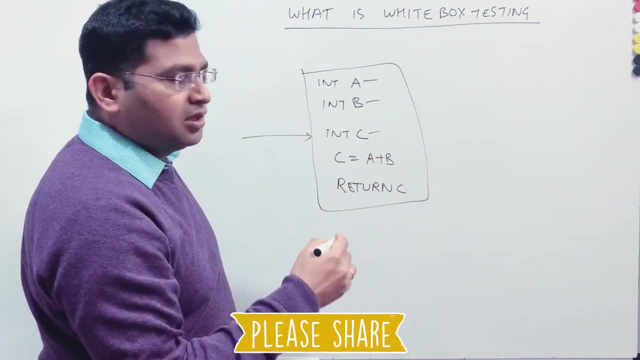 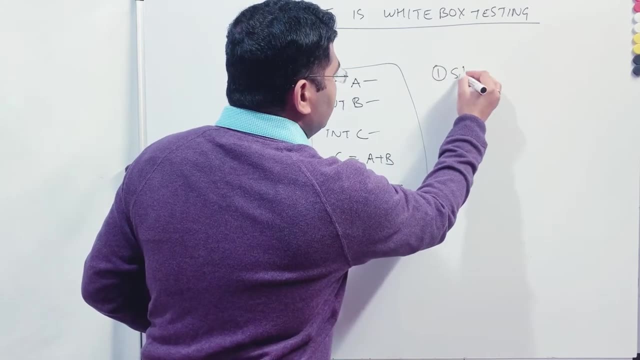 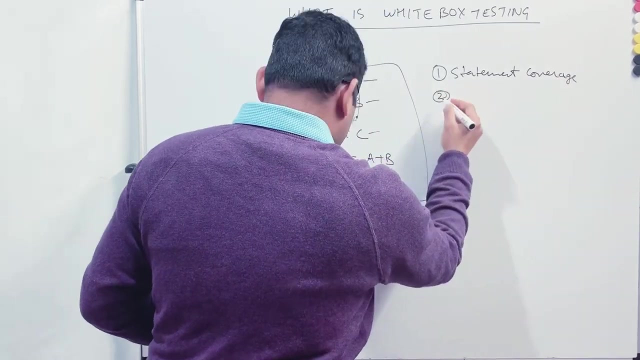 pass testing or loop testing. so all those type of testing will be part of the white box testing testing. now let me write some of those uh here as well, so that you know. so there is statement coverage and the second important one is the branch coverage. so when you verify the branch, 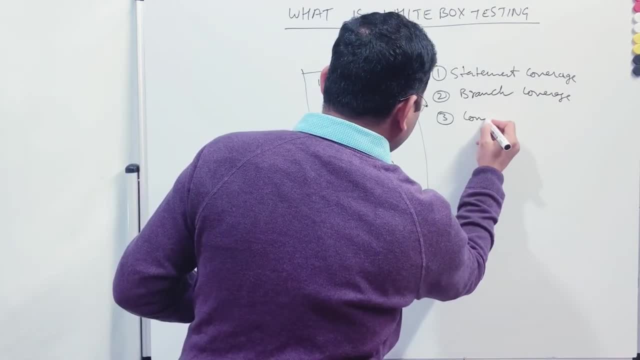 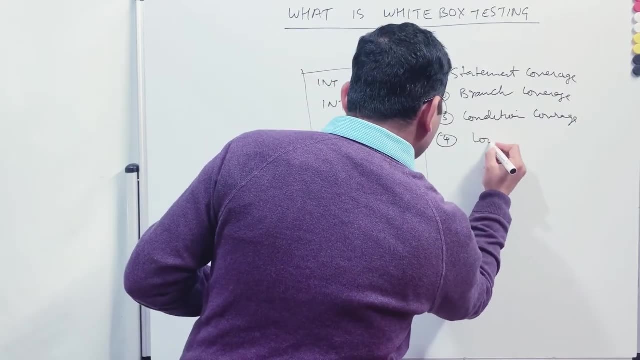 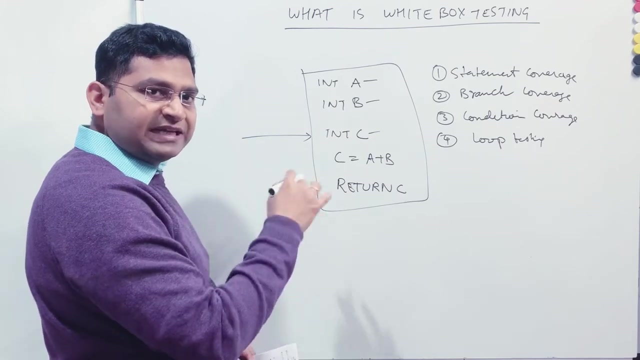 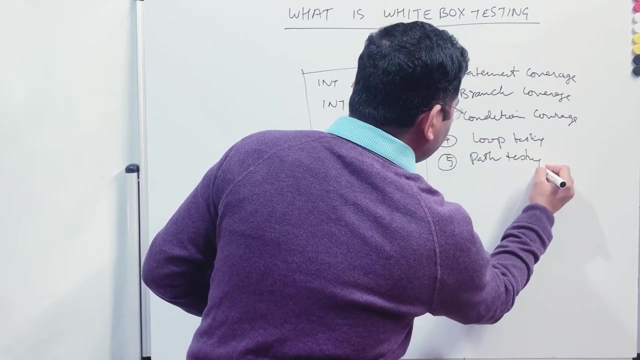 the third important one to remember is the condition coverage. then you have the loop testing, so you verify. if there are loops, different loops, then you verify all the loops are being exercised with your test cases. and then you have, you know, paths, so different path testing. if there are multiple paths, uh say, for example, you have conditions, then you verify. 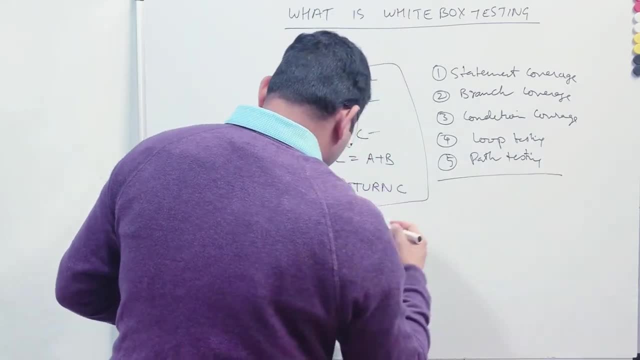 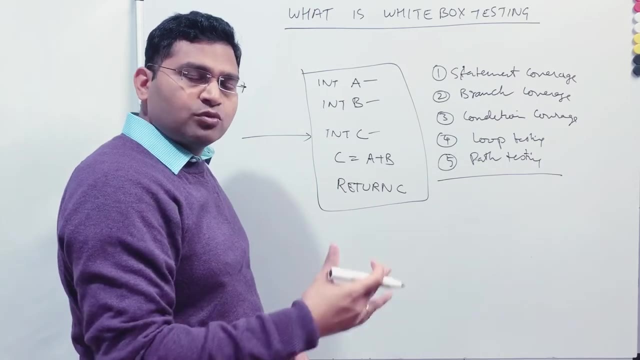 all those conditions right. so these are some of the techniques, or basically the coverage techniques, that you will verify, and there are a lot of code coverage tools available. so when you write your white box test cases, you most of the time this will be done by the developers, but as a tester, 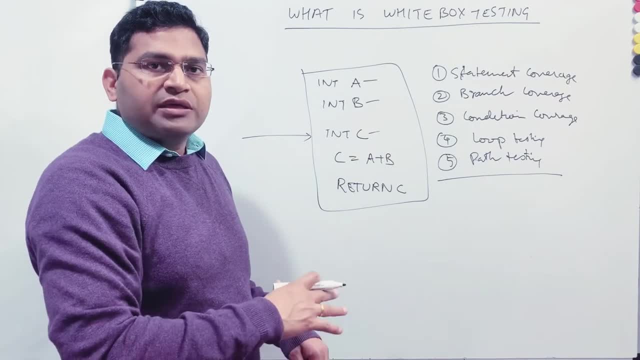 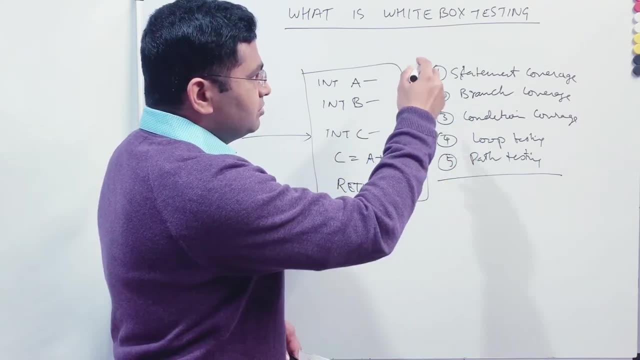 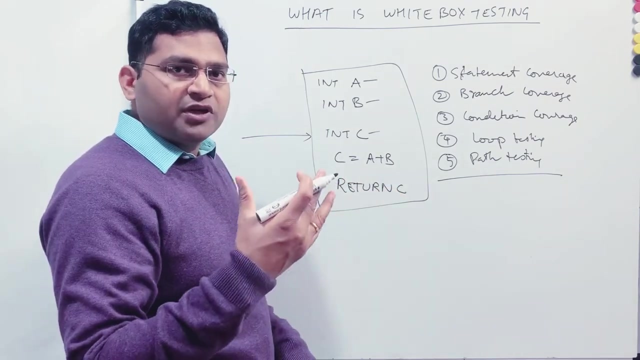 you will be required to basically provide your inputs or in case you know white box testing or need to do in your organization, then you need to cover all this. you know white box testing techniques. you need to verify that the code coverage or your test cases have uh or provide you the coverage of Statement Branch Conditions. you know loop path, all the. 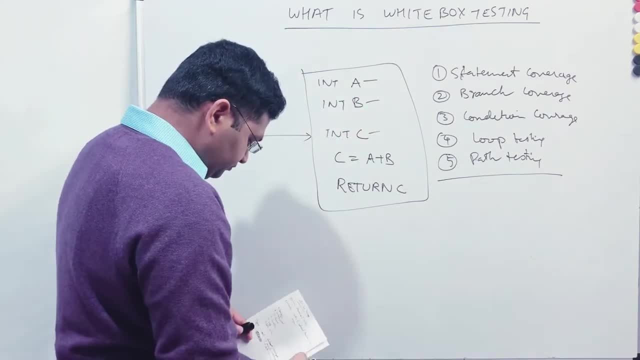 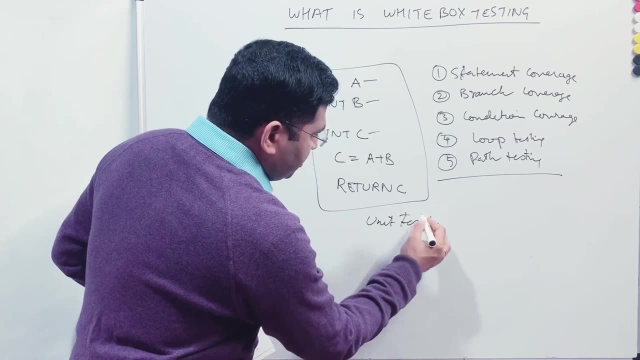 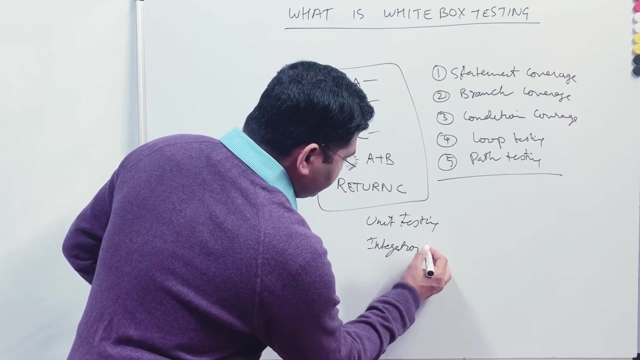 code is being exercised in the white box testing. now, usually, you know, the white box testing will happen in the unit test phase. okay, so unit testing phase is where the white box testing happens, as well as in the integration testing. okay, so integration testing it can happen in both phases. 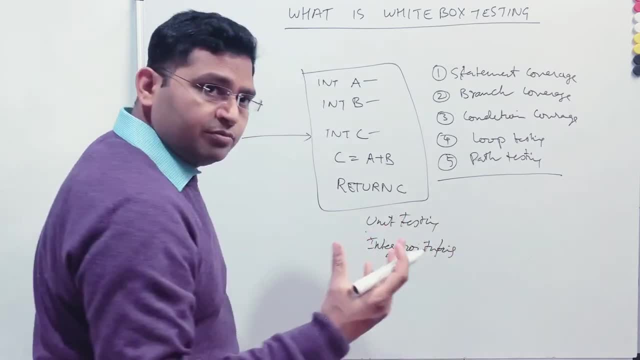 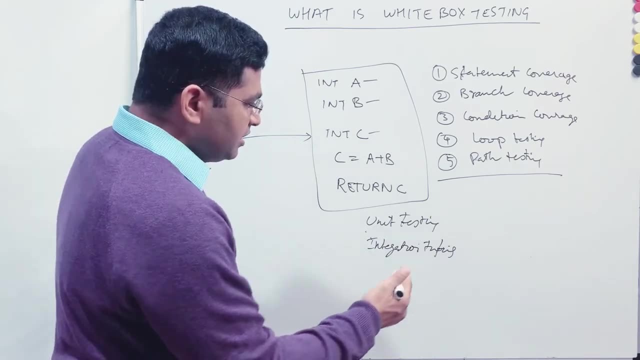 because in unit testing there will be the base testing and the integration testing. okay, so you always document in standard format. happen in both phases. because in unit testing there will be small units where- which will be you know which usually developers write the unit test cases for and there are, you know, unit test. 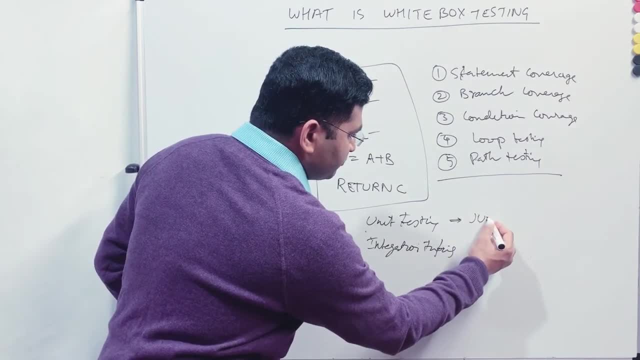 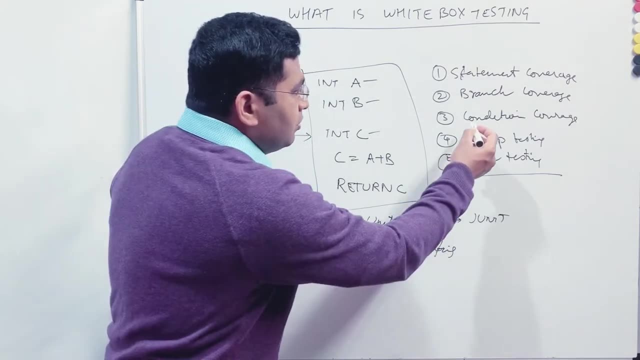 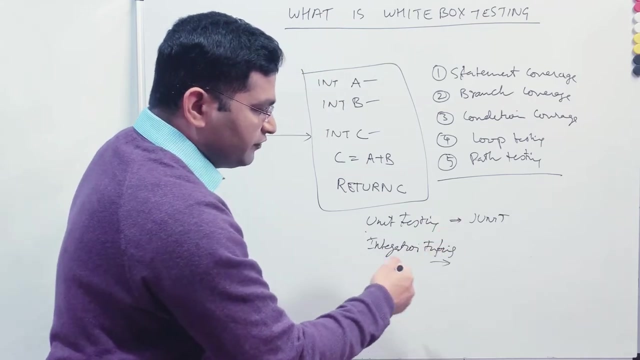 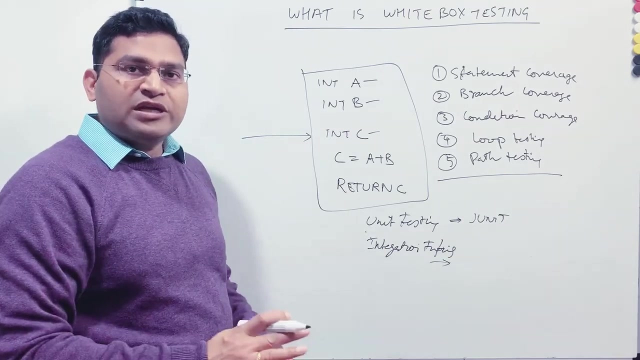 tools, for example, unit test framework- for example, j unit is very popular for java- and then integration testing. you integrate the units and make sure, after integration- all these you know statement, branch coverage, condition coverage, loop and path testing- is being done at all different levels. all right, so this is a brief about white box testing, when you have understanding and when